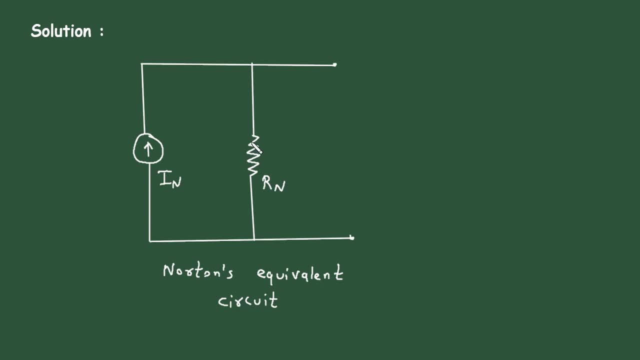 the equivalent resistance at the terminals when all the independent sources are turned off. Now, first of all, let's find the value of this Rn. So to find step number one, to find Norton's resistance Rn In the circuit, what we have to do? First of all, we will. 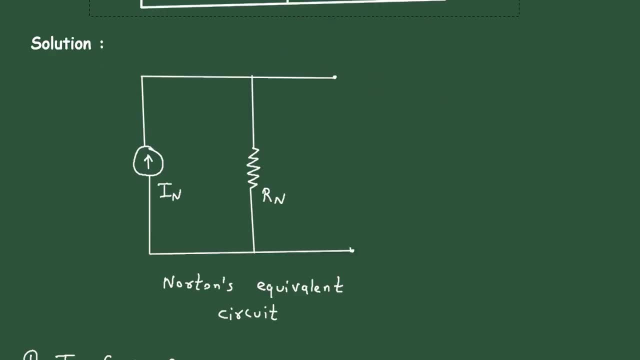 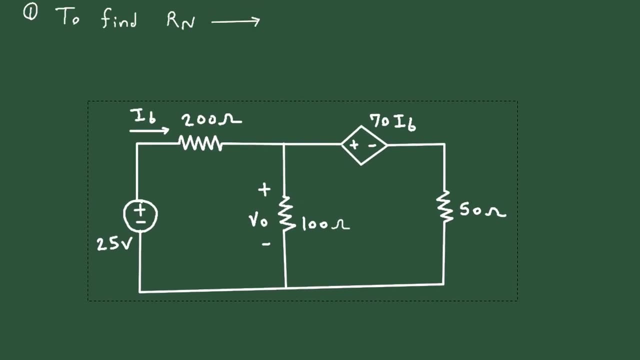 First of all, we will copy this circuit from here Now to find Rn, remove RL. this will be our first step: remove RL, and here this 100 ohm is our load register RL Now. second is: and turn off. and turn off all independent sources, turn off all independent. 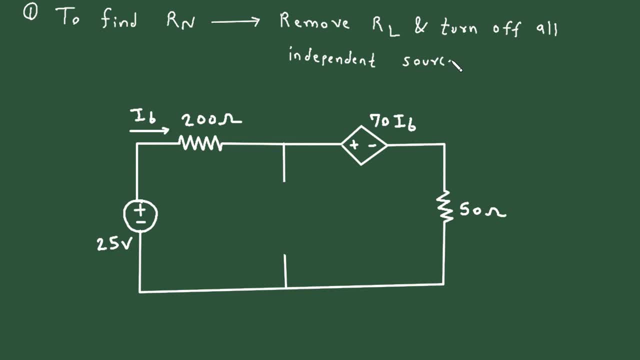 sources. As we can see here, there is only one independent voltage source, and when we turn off a voltage source, that time it will be short circuit, because we have to replace it by its internal resistance. As we can see here, it consists of a dependent source. 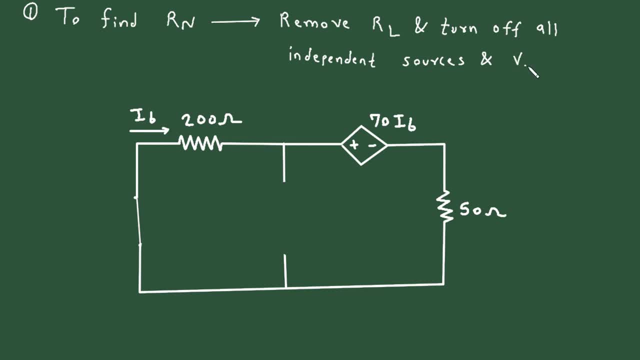 So, in case of dependent source, what we have to do? we have to consider: Vo is equal to one volt. Now, let's assume Vo is equal to one volt And here this current will be. let's say this is current Io. Now our Rth will be: Rth is equal to 1.. 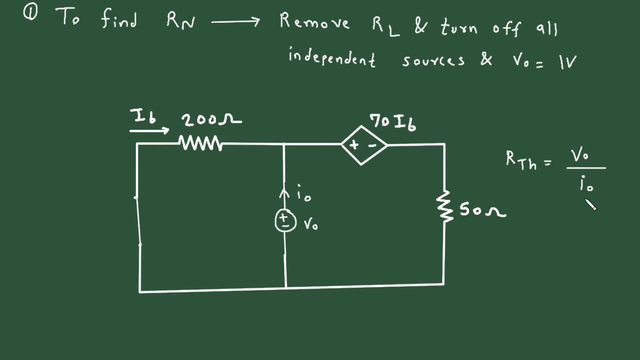 Vo upon Io, voltage divided by current. here the value of voltage is one volt. we are assuming Vo is equal to one volt, So one upon Io. now to find the value of Rth, we have to find the value of Io. So let's find the value of Io. 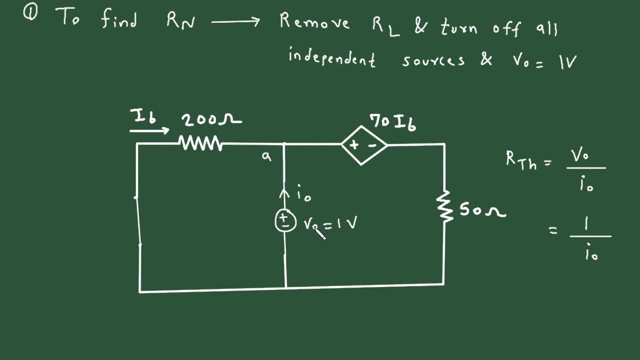 Let's say this is a node A and, as we can see here, this voltage will be Vo and Vo is equal to one volt. So this voltage will be one volt. Let's say this is current I1,, this is current Io and this is current I2.. 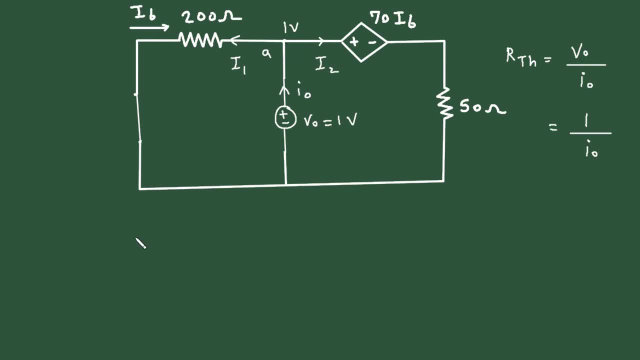 Now what we will do. we will apply KCL at node A. We are solving this problem by using nodal analysis. In case of nodal analysis, we use KCL. So apply KCL- that is Kirchhoff's current law- to node. 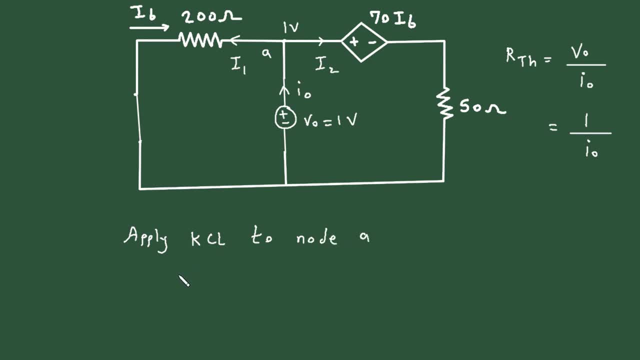 According to Kirchhoff's current law, summation of current in is equal to summation of current out. That is, summation of all the currents entering a node is equal to summation of all the currents leaving the node. Here the entering current is Io. 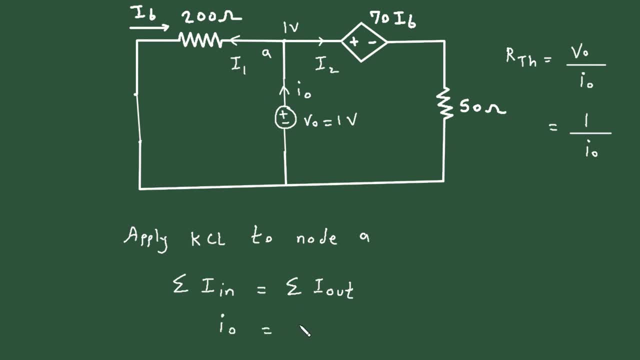 So Io is equal to leaving. currents are I1 plus I2, I1 plus I2.. Now this I1 will be Vo, I1 will be 1 minus 0.. Let's say this is a reference node, So 1 minus 0 divided by 200. 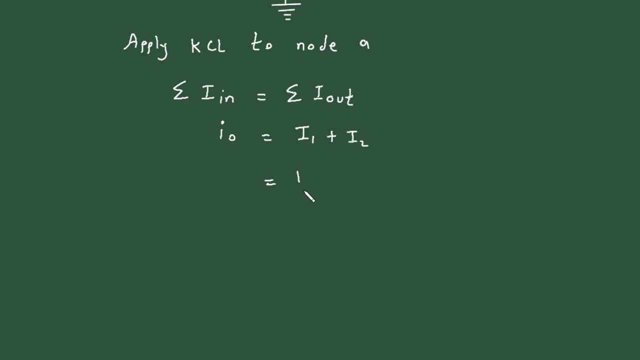 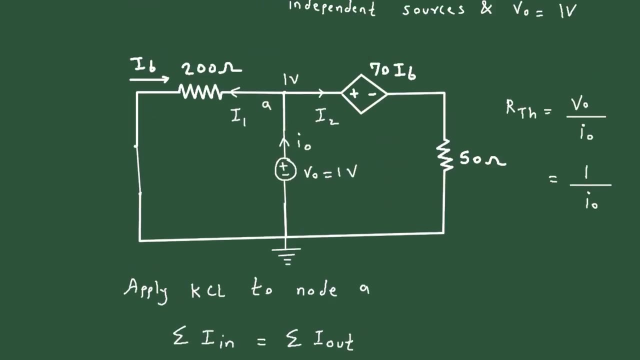 1 minus 0, or simply 1 minus 0 divided by 200.. Io is equal to, and plus 1 minus 0 divided by 200.. This will be the value of I1 and then I2.. So I2 will be I1.. 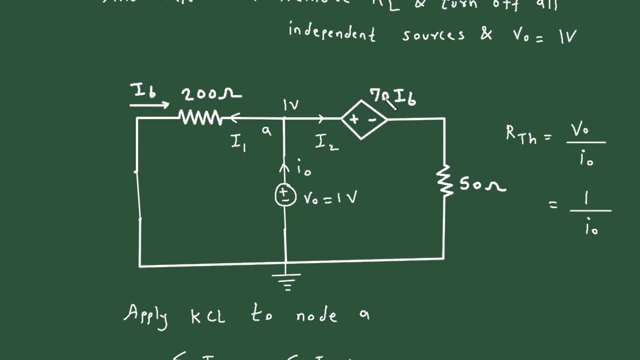 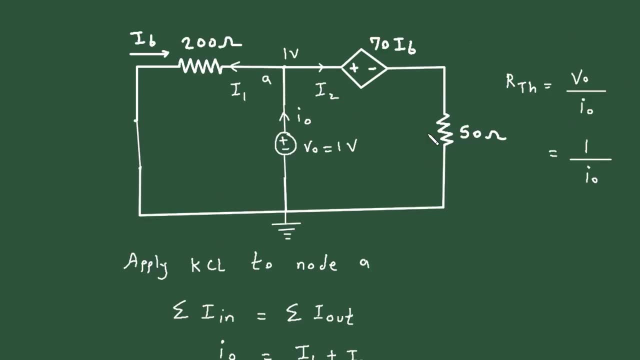 I2 will be I1.. I2 will be I2.. I2 will be I1.. I1 minus 70 Ib. I1 minus 70 Ib minus 0.. So minus 0, we will skip it divided by 50 ohm. 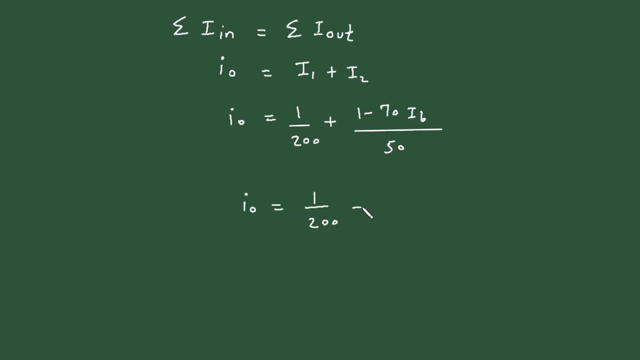 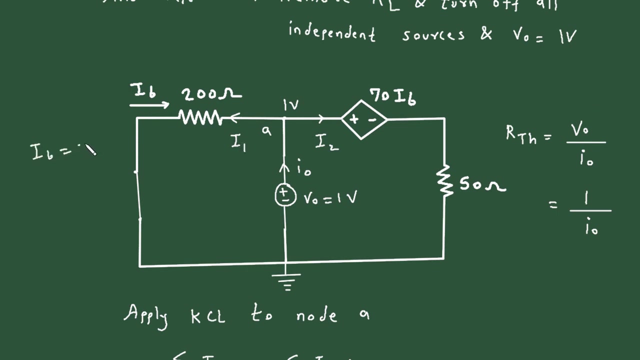 Now this will be: I0 is equal to I1 upon 200 plus I1 upon 50 minus 70. So this is a reference: 70 by 50.. Now, here in place of this, IB. as we can see here, IB is equal to IB is equal. 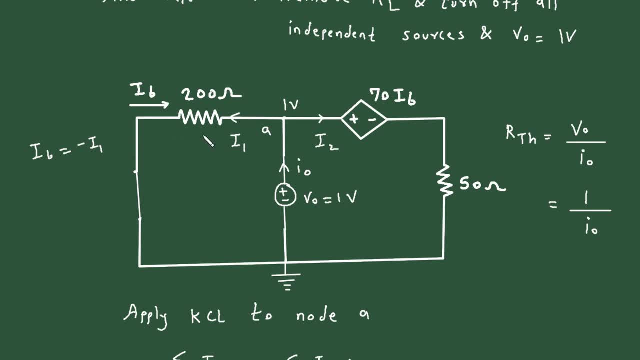 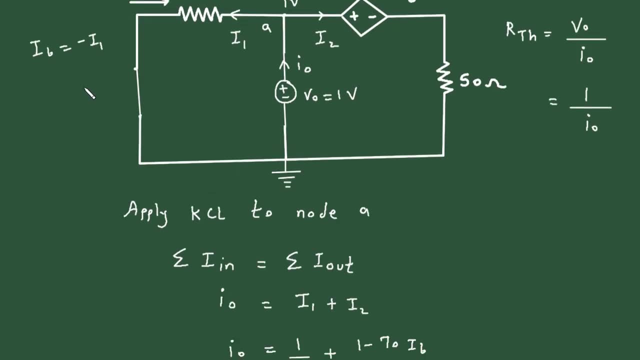 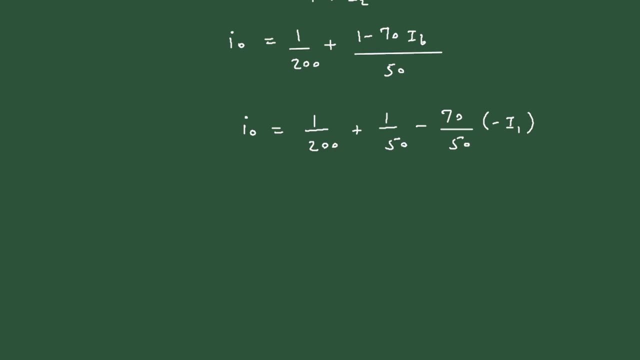 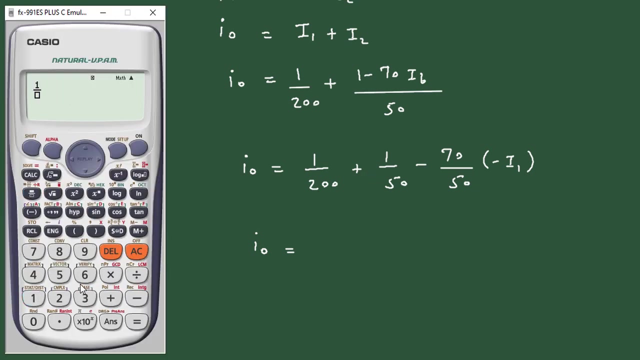 to minus i1, because the both the directions are opposite. IB and i1 direction is opposite. So this will be: IB is equal to minus i1. So this will be minus i1.. Now again we can further simplify this. So IO is equal to one by 200 plus one by 50, one by 200 plus one. 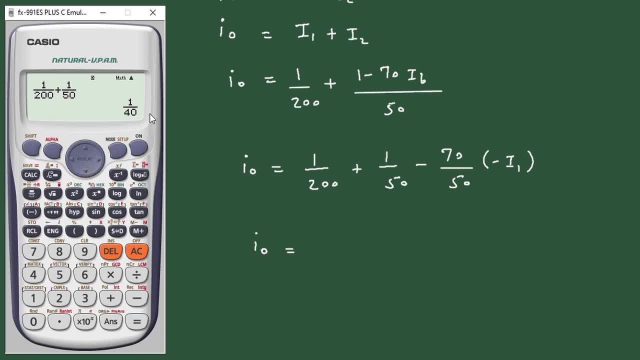 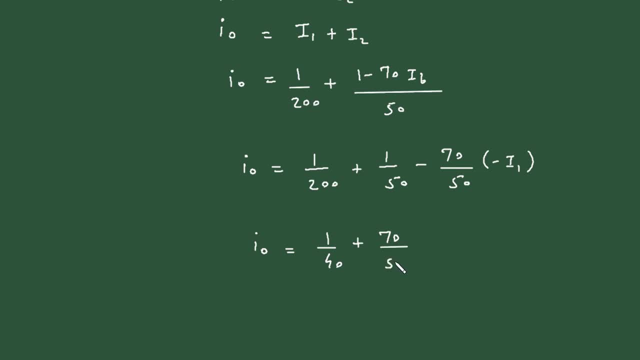 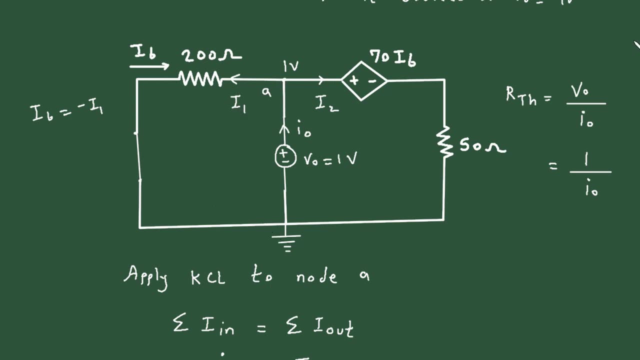 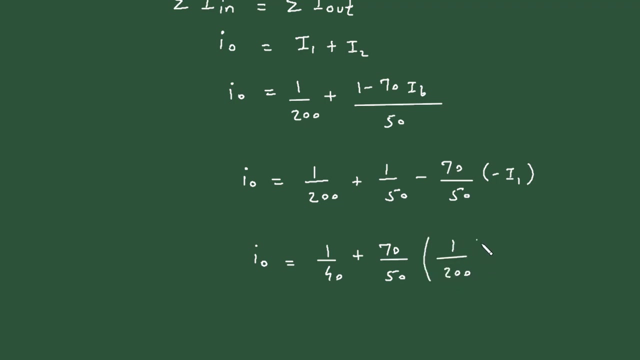 by 50.. So it is one by 40, one by 40, and this will be minus minus plus 70 by 50. And this is i1. So this will be: i1 is equal to 1 minus zero divided by 200.. 1 minus zero divided. 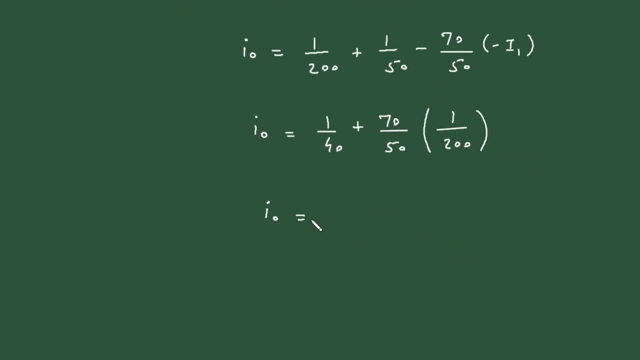 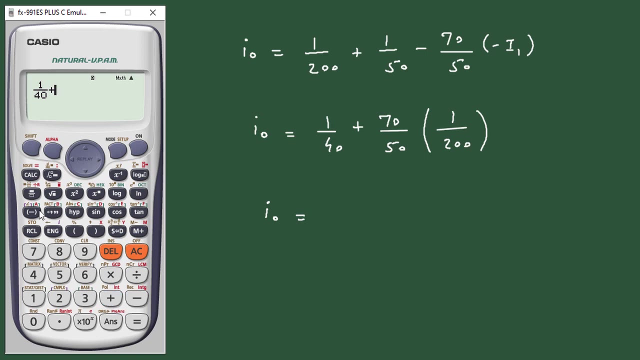 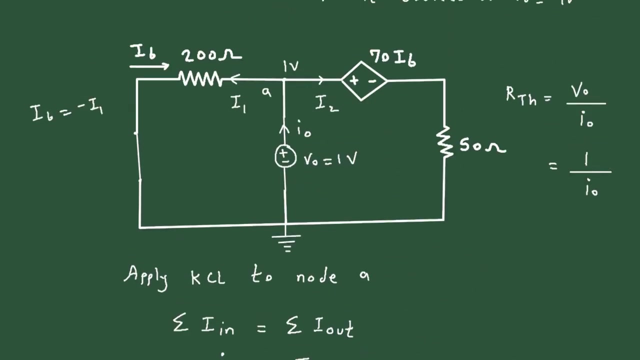 by 200.. So IO is equal to This way will be 1 by 40 plus 70 by 50 into 1 by 200, so it is 0.032, 0.032 since it is current. so its unit will be ampere. but we have to find rth and rth is equal to 1. upon io, rth is equal. 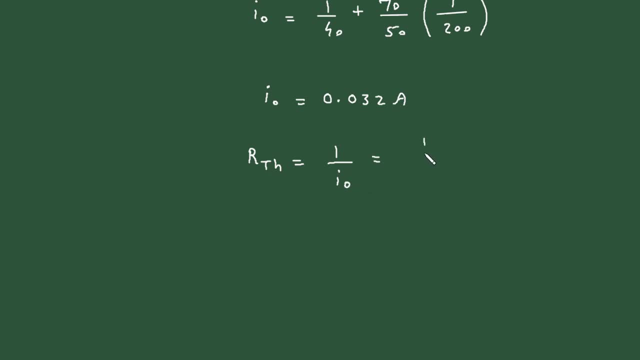 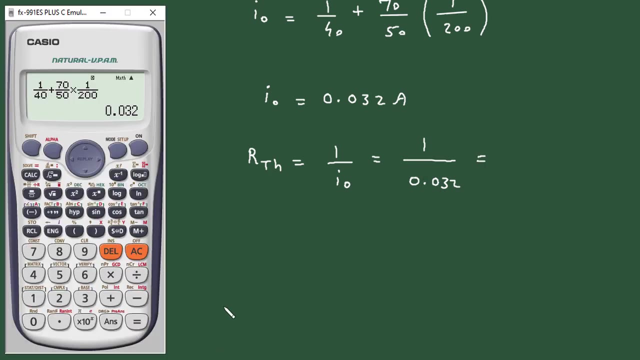 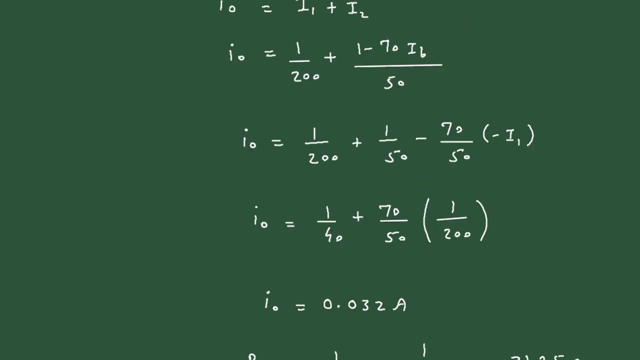 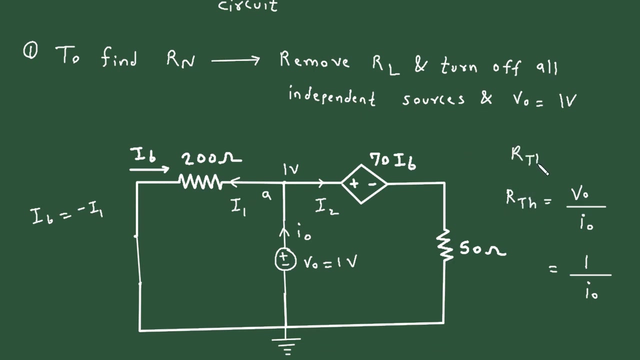 to 1 upon io, so this will be 1 upon 0.032. now, this will be 1 upon answer, so it is 125. or we can write 31.25.. 31.25 ohm. this is not the value of rth. also we can say rth is equal to rn. but here we 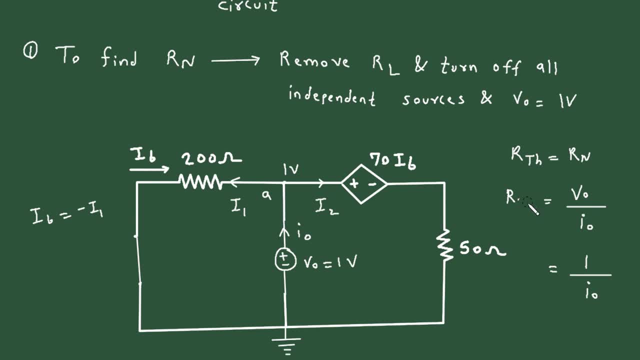 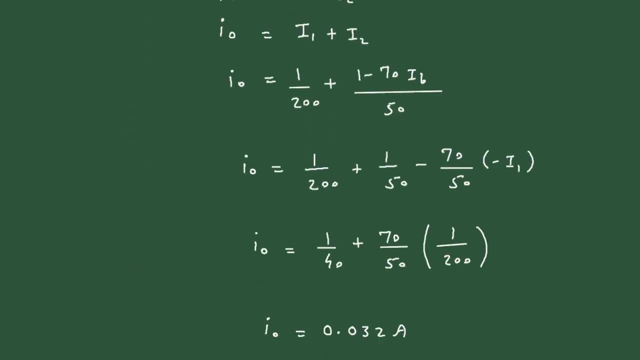 are solving for norton's theorem. so here we have to write rn. this is norton's resistance rn, because we are finding rn, and here also this will be norton's resistance rn. so this is norton's resistance rn. so rn is equal to 31.25 ohm. also remember that thevenin's resistance 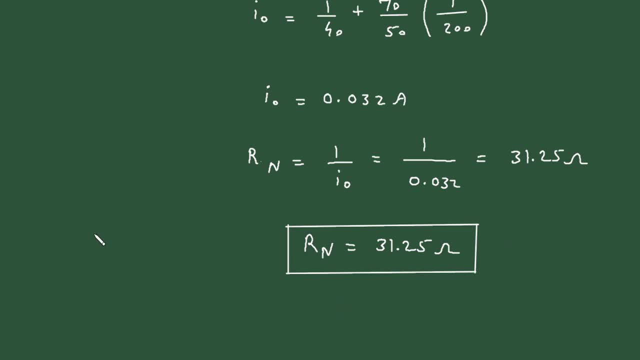 is equal to norton's resistance. that is here we can write note: rth is equal to rn. now, next is we have to find the value of rn. so we have to find the value of norton's current in. so step number two, to find in again what. 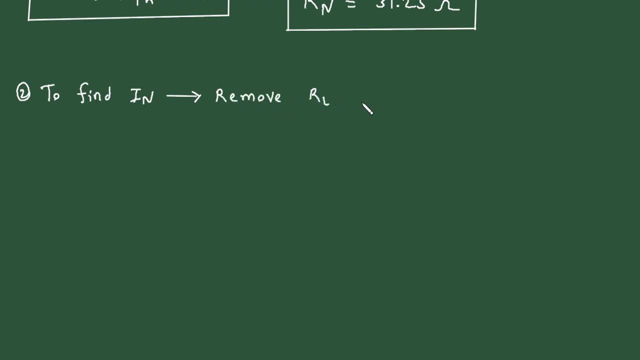 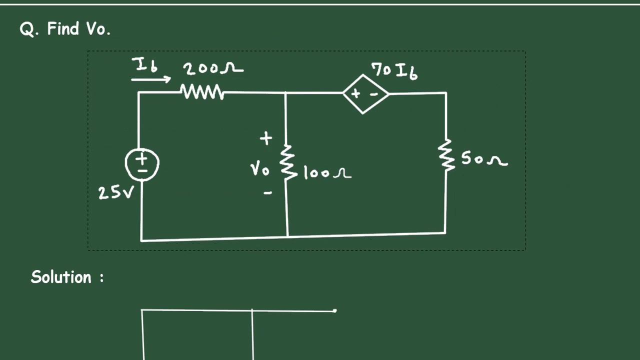 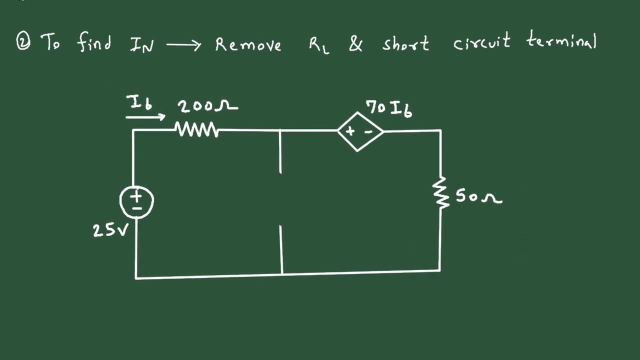 we have to do: remove rl and short circuit terminals. so let's copy this circuit from here directly. and what we have to do, we have to remove rl. so let's remove this rl from here and then short circuit this terminals. now this will be our norton's current in. let's say this: 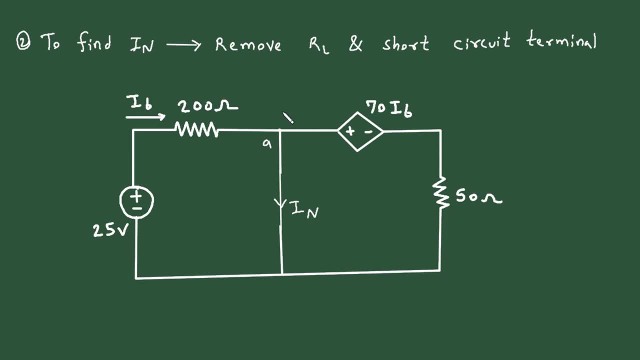 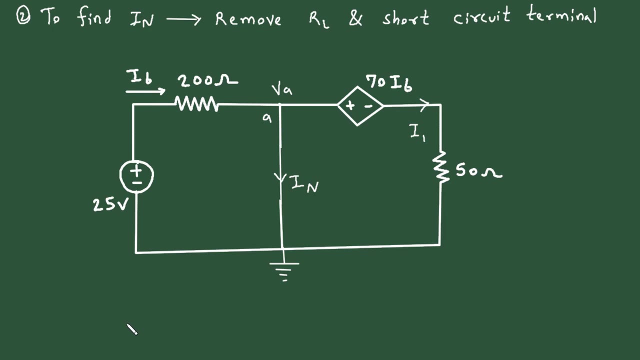 is a node a and let's say it's voltage is va. let's say this is a reference node. let's say this is a current i1.. Now we will apply KCL at node a, apply KCL, that is Kirchhoff's current law- at node a. 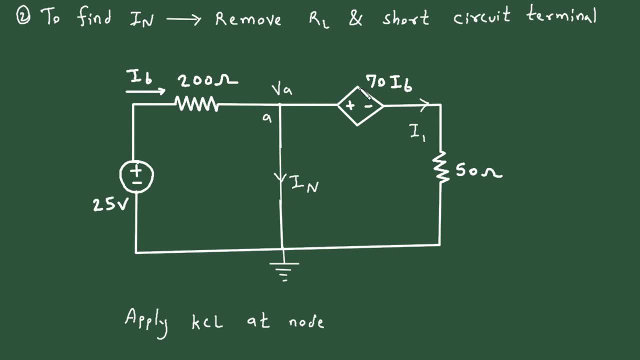 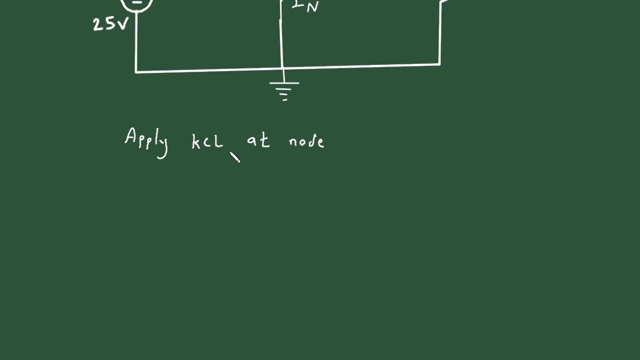 to find the value of this IN. we have to find this IN and we are finding this by using KCL or nodal analysis. So KCL stands for Kirchhoff's current law. according to KCL, summation of current in is equal to summation of current out. at this node, entering current is IB. 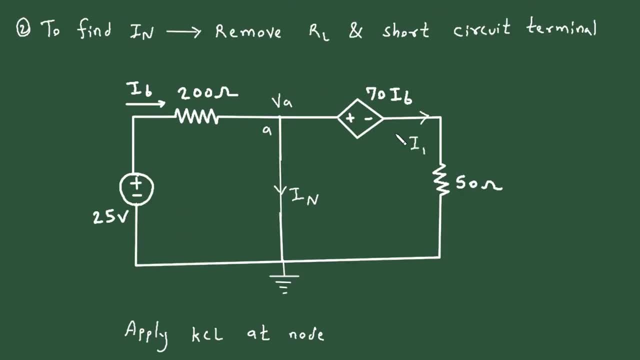 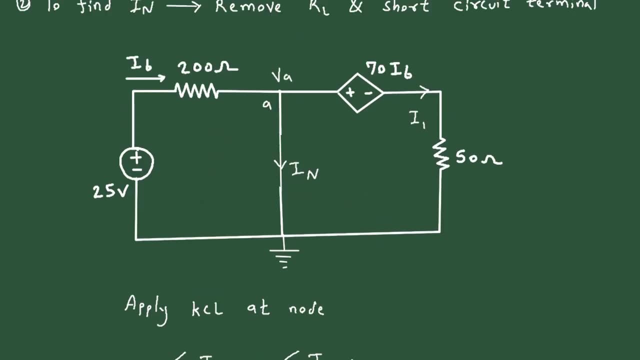 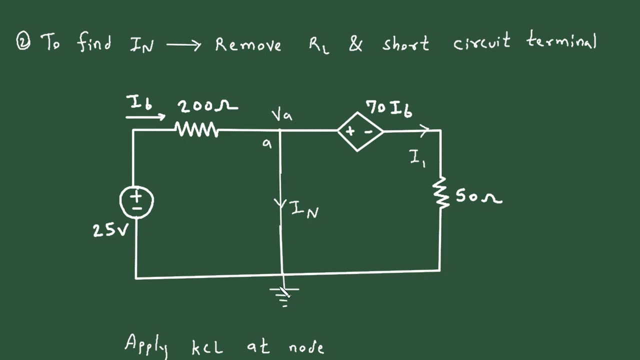 So IB is equal to leaving current. leaving current is i1 plus iN. i1 plus iN. Now IB in voltage form will be 25 minus VA, and here we can see VA is connected to ground, So its voltage will be zero. 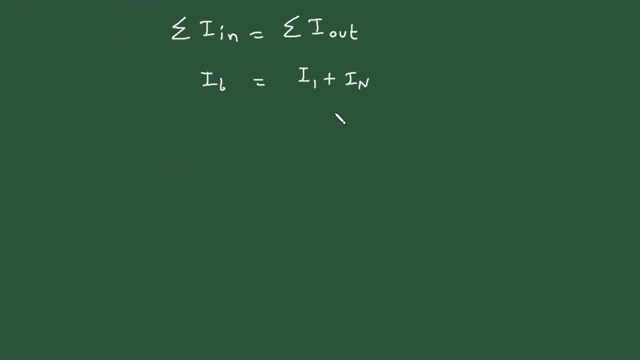 So 25 minus zero divided by 200. 25 minus zero divided by 200 is equal to i1.. Now i1 will be zero. Then zero minus 70 IB, Zero minus 70 IB, 70 IB divided by zero minus 70. IB minus zero divided by 50 ohm plus iN. this iN as it is. 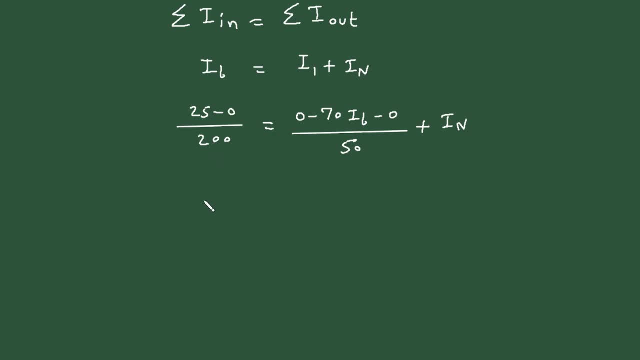 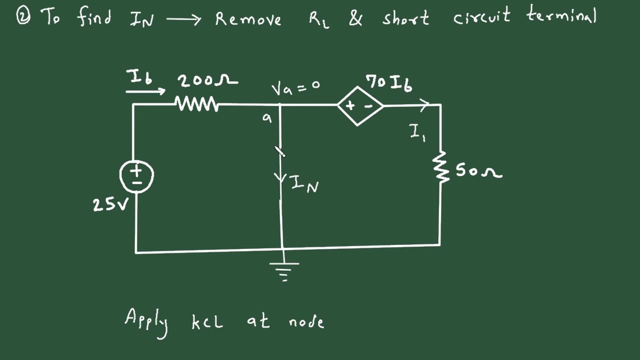 Now, if we solve this, so it will be 25 divided by 200, so it will be 0.125 is equal to, and this will be minus 70 by 50, now IB in voltage form. again, this will be 25 minus zero divided. 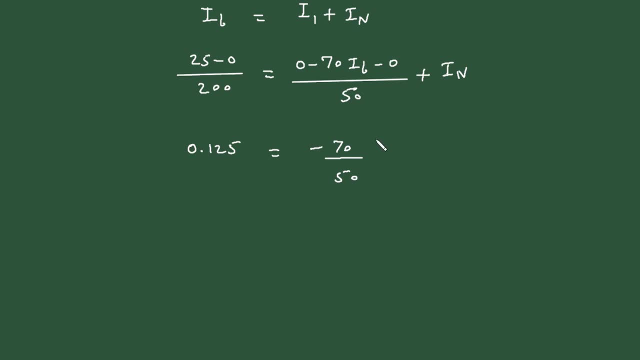 by 200, 25 minus zero divided by 200, then plus iN, now this will be 0.125- is equal to minus 70 by 50. So this will be minus 70 by 50 and minus 70 divided by 20.. 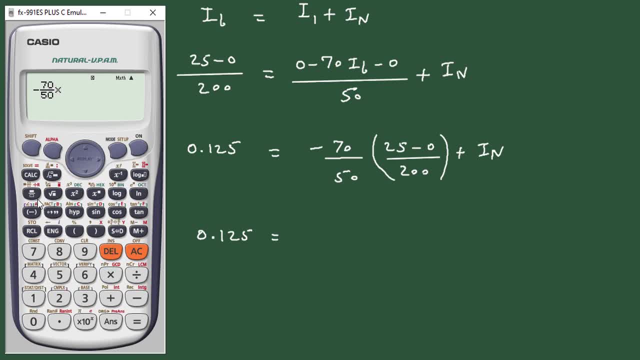 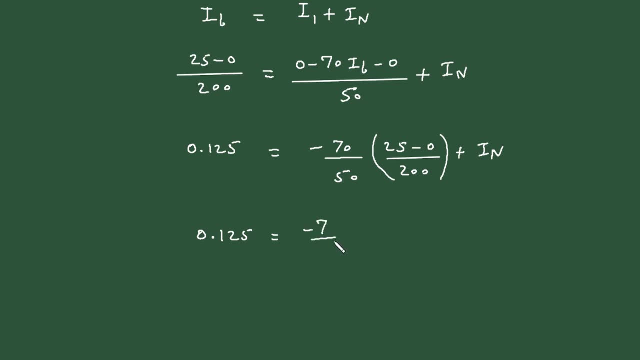 Minus 70 divided by 50 into 25. minus 70 divided by 50 into 25 by 200. so it is minus seven by 50. so it is minus seven by 40, minus seven by 40 plus iN, if we take this on this side. 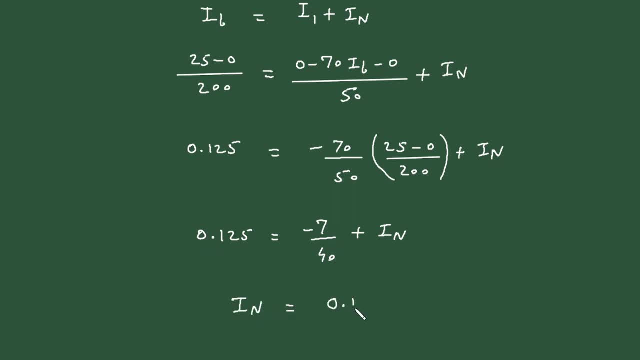 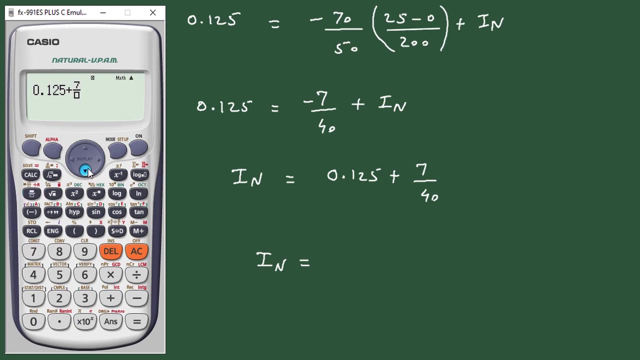 So it will be like iN is equal to zero point one, two, five. So it will be like iN is equal to 0.125.. So it will be like iN is equal to 0.125.. plus seven by 40. So therefore, I n is equal to 0.125 plus seven by 40. So it is 0.3.. 0.3. 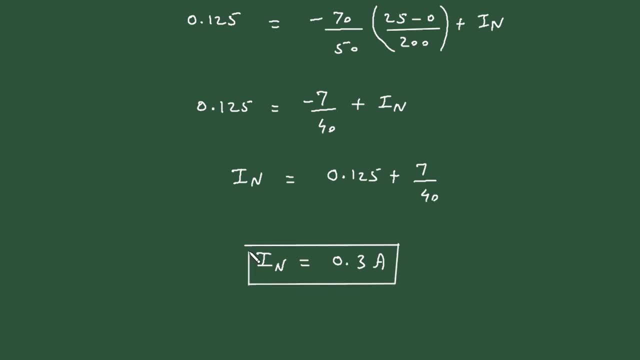 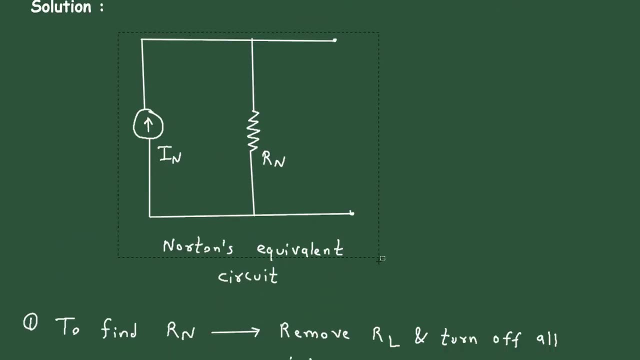 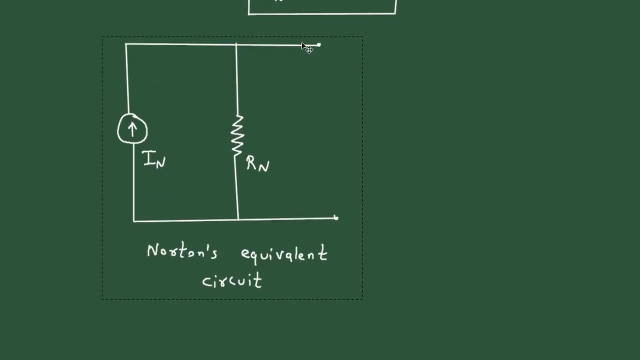 since it is current, so its unit will be ampere. Now we can draw Norton's equivalent circuit, So we will directly copy it from here And then substitute the value of Norton's current. It is 0.3 ampere. The value of Norton's resistance is 31.25 ohm. 31.25 ohm And here this will: 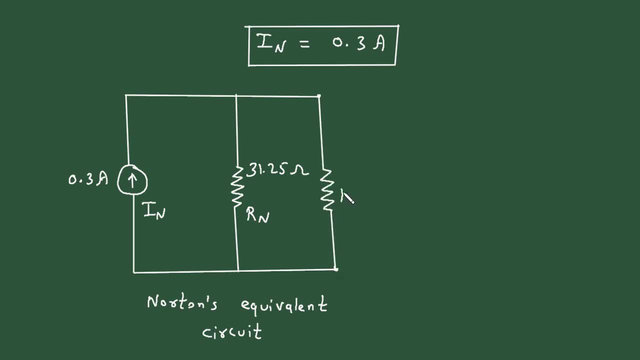 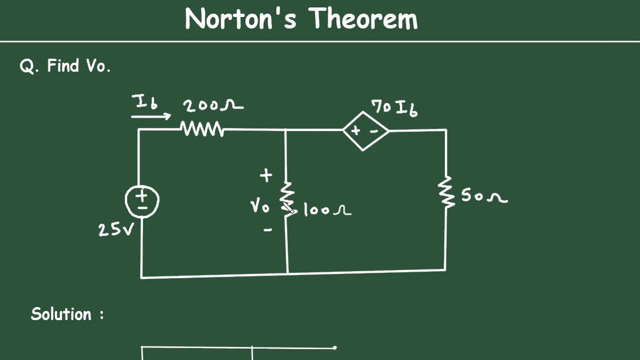 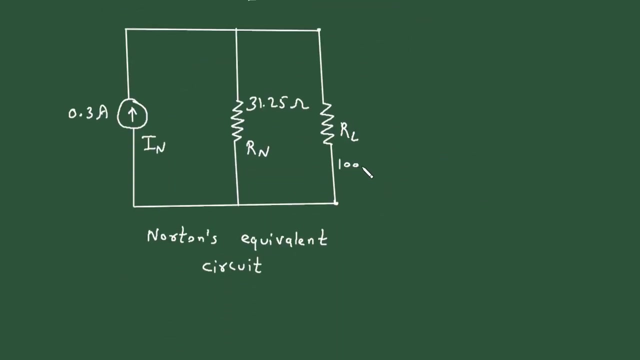 be our load resistor RL. The value of load resistor RL is 100 ohm And the voltage across is VO. So this is 100 ohm And voltage across is VO And let's say this current is IL. So let's find IL, IL is. 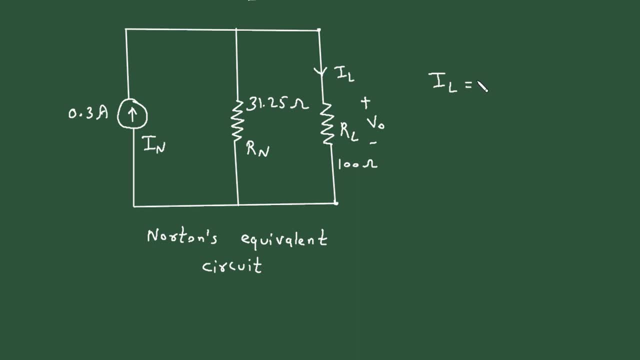 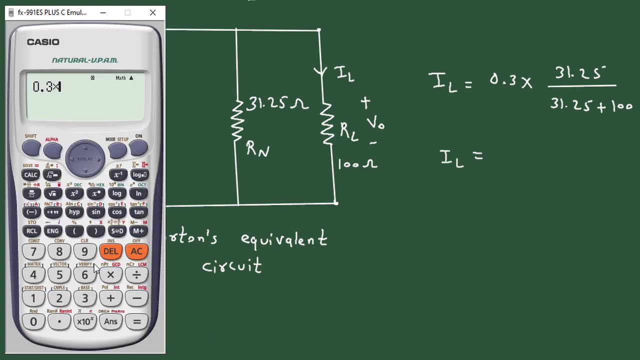 equal to. according to current division rule, IL is equal to 0.3 multiplied by opposite branch resistance, that is 31.25 divided by 31.25 plus hundred. So IL is equal to 0.3 multiplied by 31.25, divided by 31.25 plus. 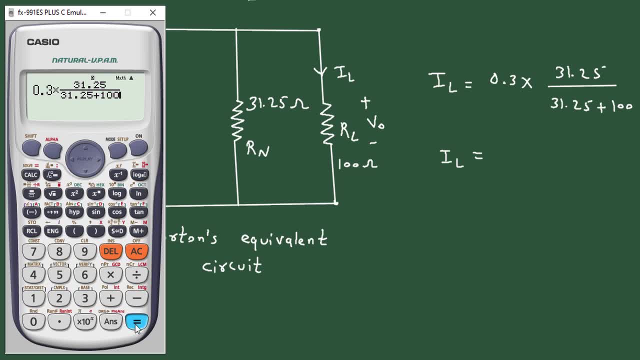 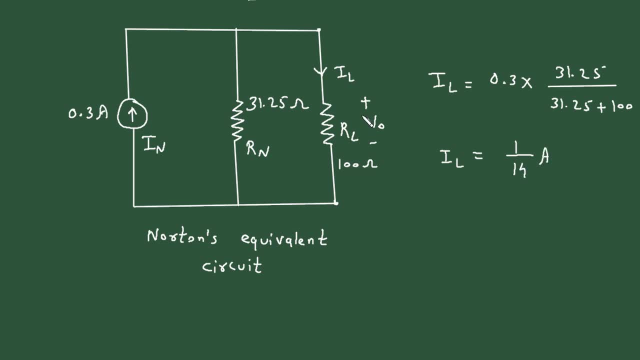 100.. So it is 1 by 14. 1 by 14 ampere is the value of IL, but we have to find VO and VO is equal to IL multiplied by RL. the value of IL is 1 by 14, multiplied by resistance value is. 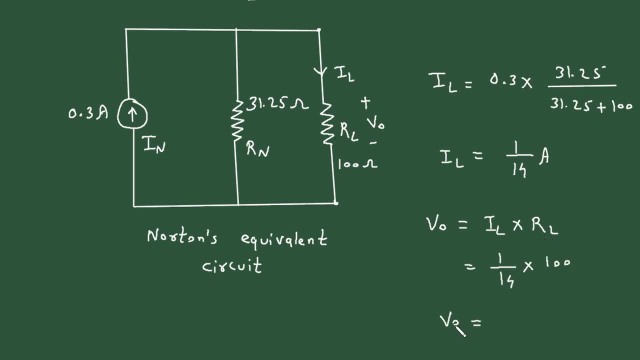 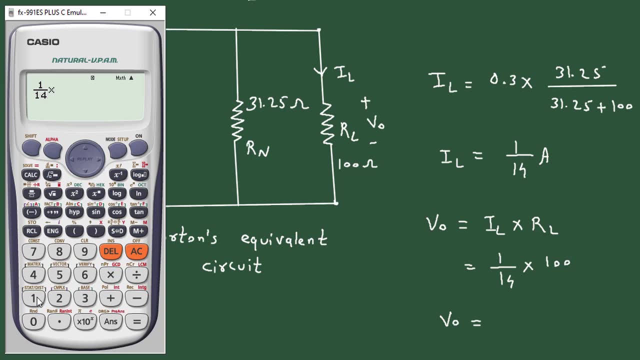 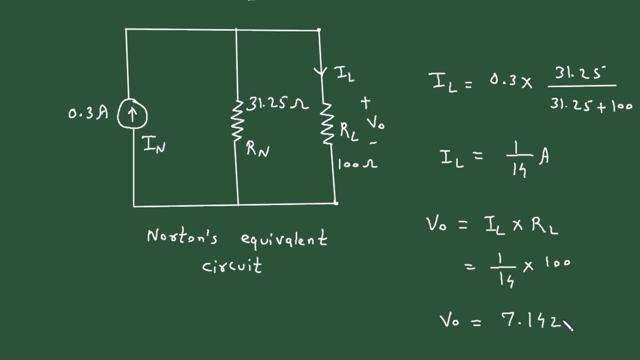 100, so VO is equal to 1 by 14 multiplied by 100, so it is 7.142. 7.142 since it is a voltage, so its unit will be volts. so this is the answer for VO. this is our final answer by using Norton's. theorem. Thank you.